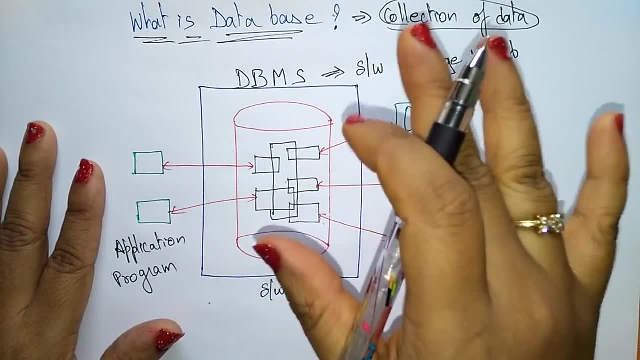 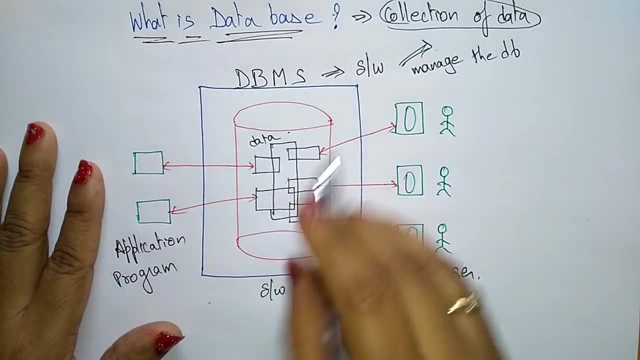 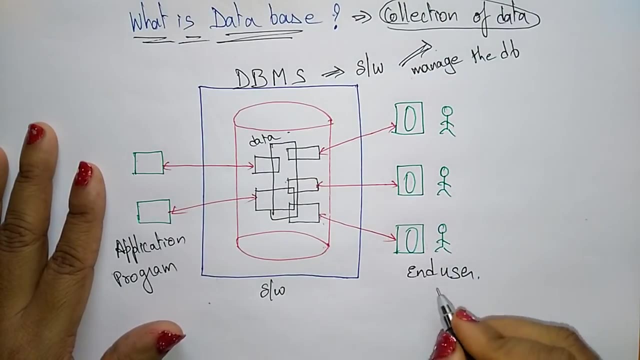 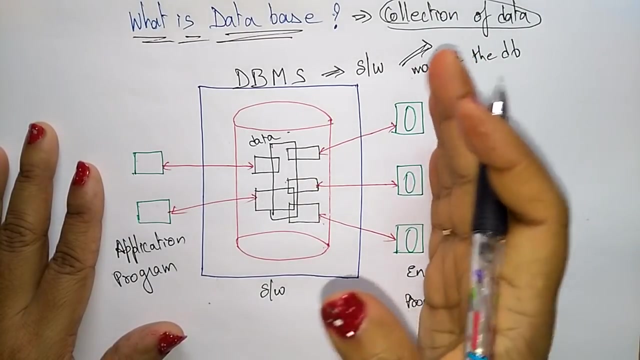 the database management system. with the help of this software, we are storing a data. So this is all a data. Okay, So this data will access by the users, the end users. So end users, or the programmers or the administrators, means we are the users, We want to access the data. So how we can access this data, We can access the data. 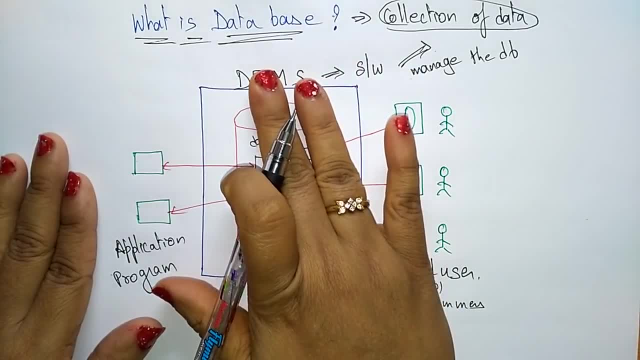 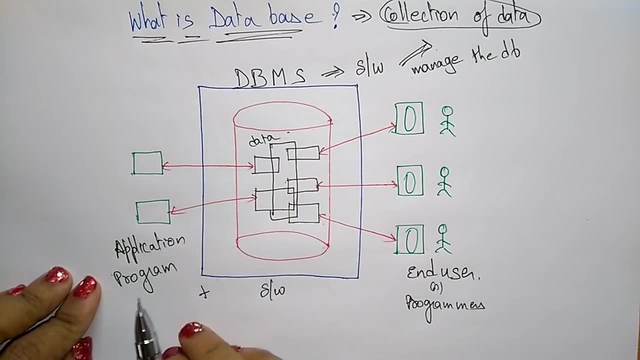 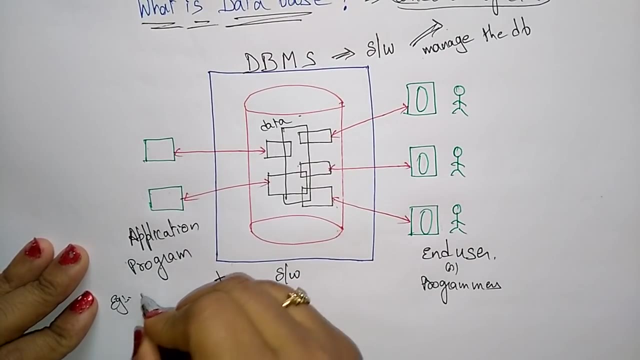 Only with the help of database management system means that with the help of the software and the application program, So what you call this application program, application programs, or nothing but like C, C plus plus Java, So these are all the different application programs. So with the help of these application programs we are accessing the data. 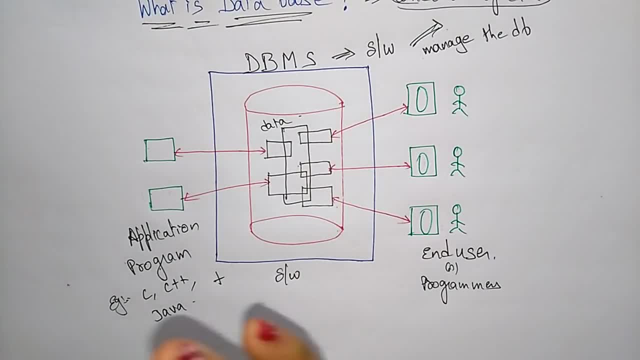 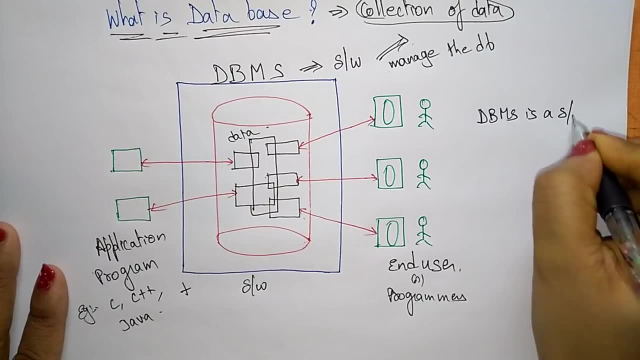 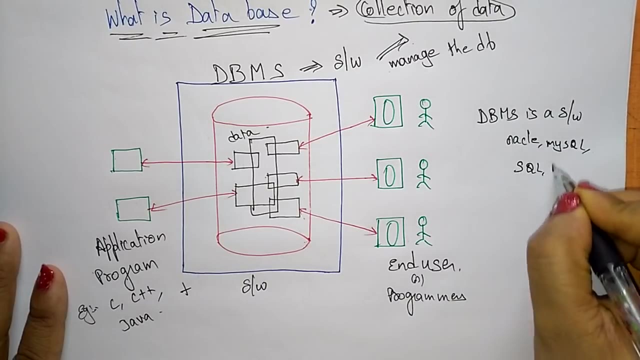 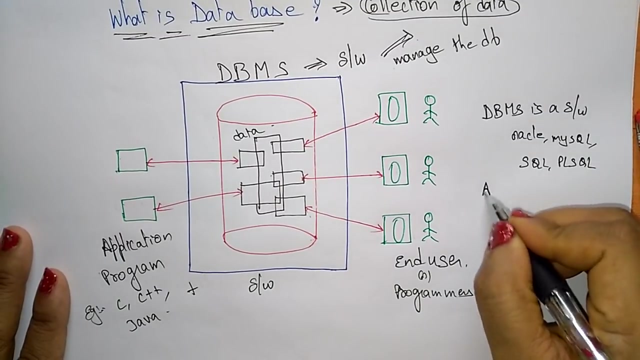 From the database management system. Okay, So don't be confused. Actually, database management system is a software, means Oracle, MySQL, SQL, PL, SQL. So these are all the different database management system software. and coming to the application program, application program. So nothing but C. 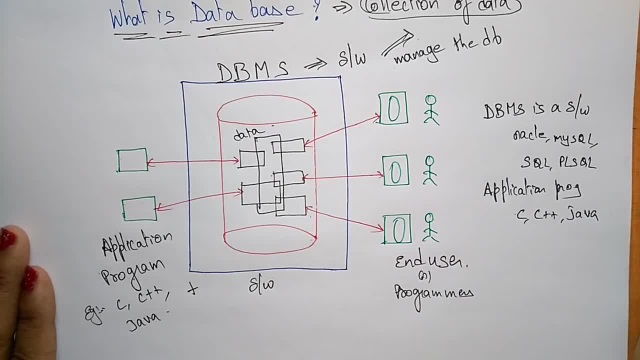 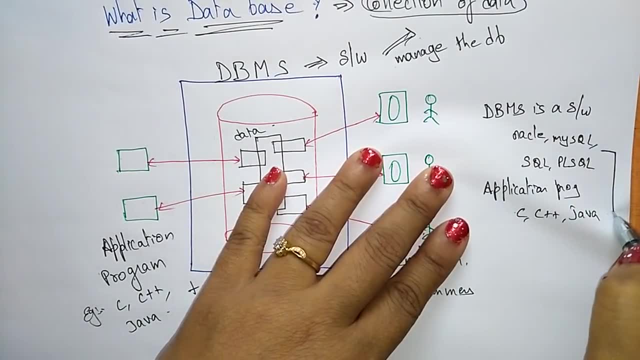 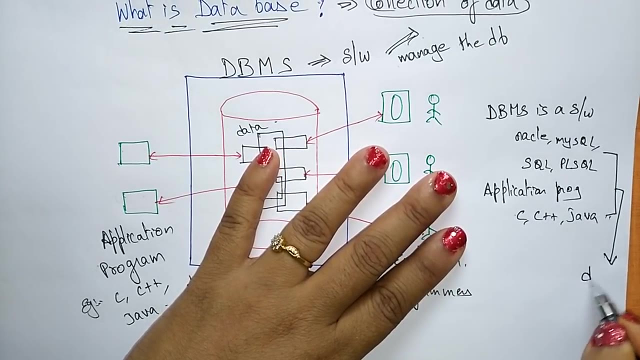 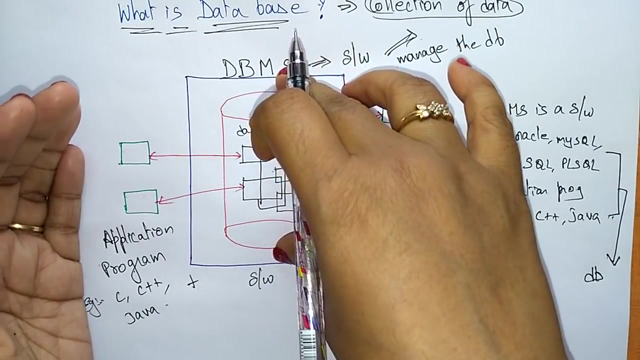 C plus plus Java. So these are all the application program. Okay, So with the help of these application program and database management system software, we are storing the data in a database. Okay, So here this is a software. with the help of this application program and the software, the data will store. 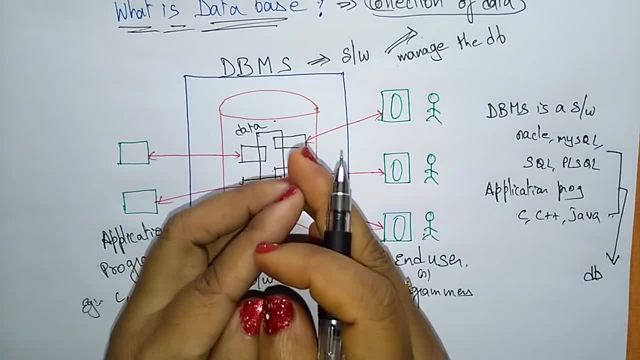 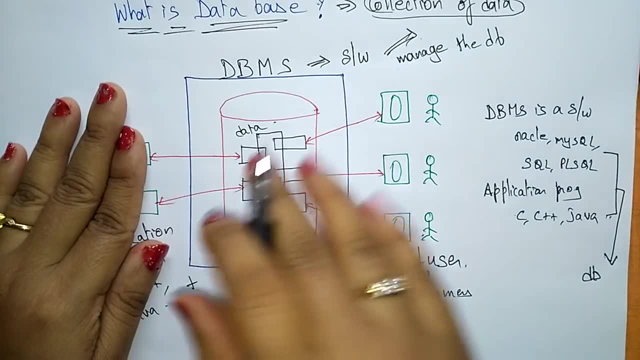 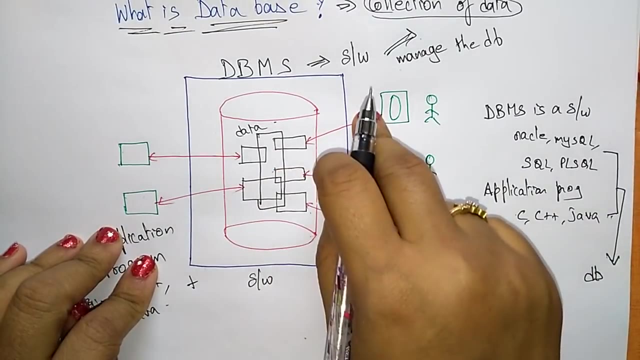 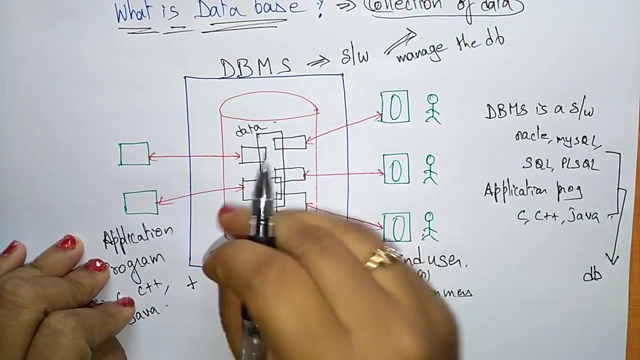 So we can access. means the end user can access these data with the help of application programs and the database management system software. So with the help of this software and the application program, we can access the data. means we can retrieve the data, We can access the data, We can modify the data.